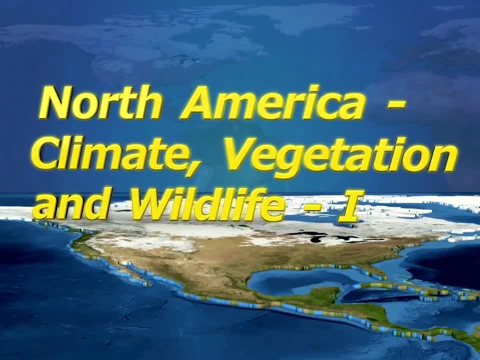 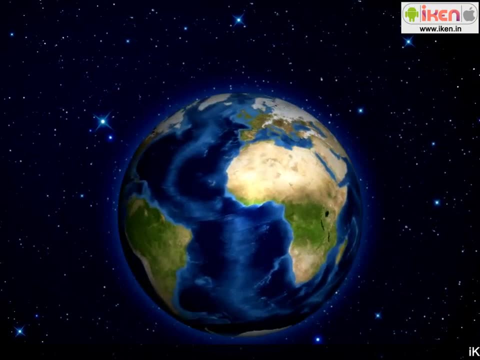 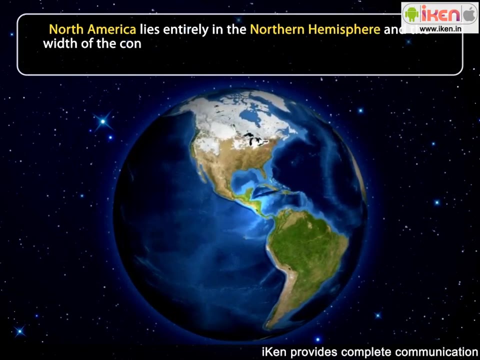 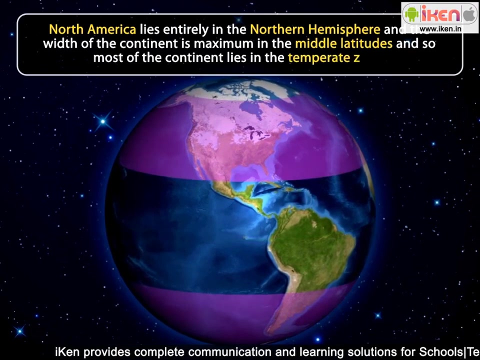 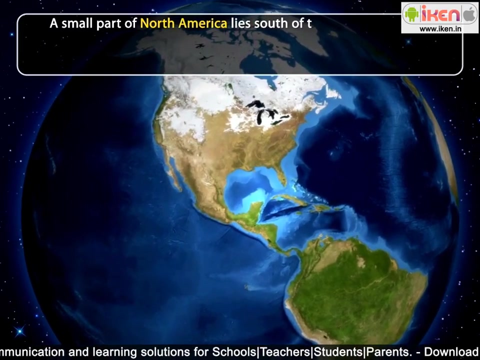 North America: Climate, Vegetation and Wildlife. Part 1: North America lies entirely in the northern hemisphere, and the width of the continent is maximum in the middle latitudes, and so most of the continent lies in the temperate zone. A small part of North America lies south of the Tropic of Cancer, Southern Mexico. 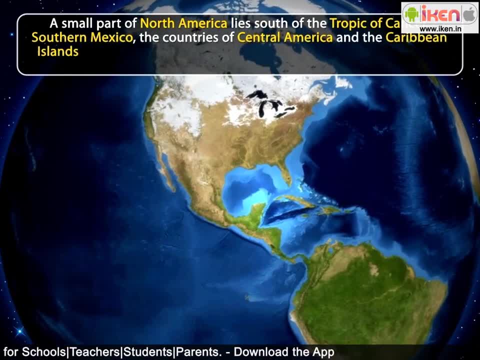 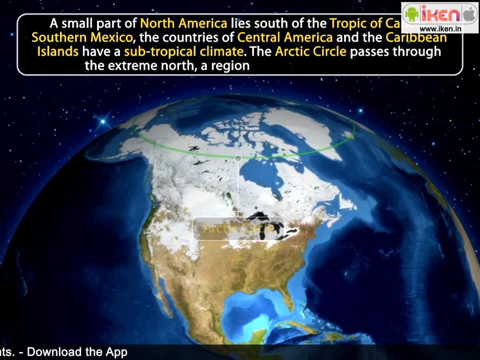 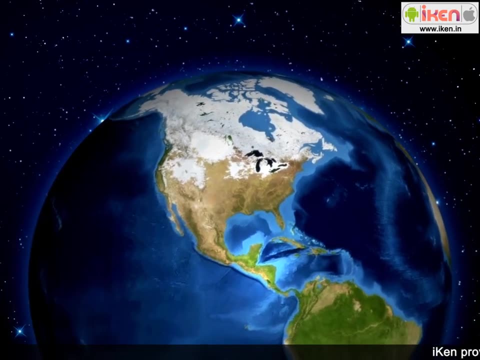 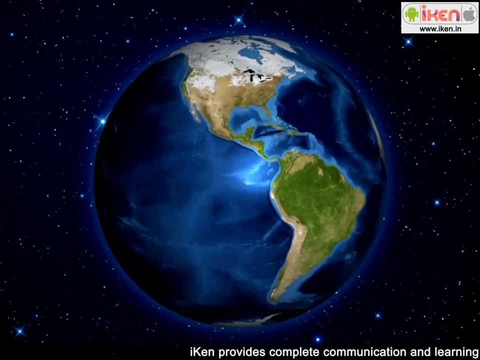 passes through the extreme south, a region which is extremely cold. The continent passes through the extreme north, a region which is extremely cold. The continent passes through the extreme south, a region which is extremely cold. The continent passes through the extreme north, a region which is extremely cold: The continent. 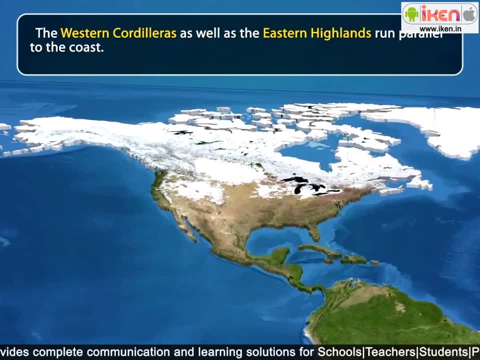 passes through the extreme south, a region which is extremely cold. The continent passes through the extreme north, a region which is extremely cold. The continent passes through the extreme south, a region which is extremely cold. The continent passes through the extreme north, a region which is extremely cold: The continent. 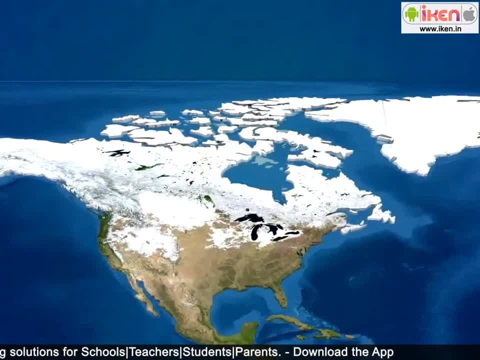 passes through the extreme south, a region which is extremely cold. The continent passes through the extreme north, a region which is extremely cold. The continent passes through the extreme south, a region which is extremely cold. The continent passes through the extreme north, a region which is extremely cold: The continent. 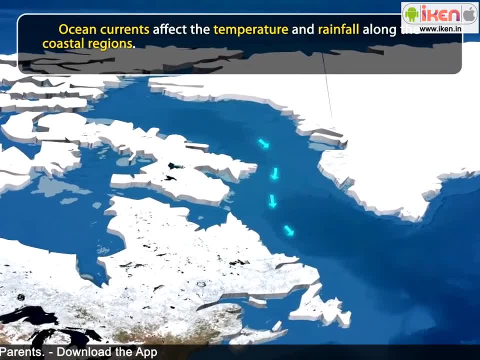 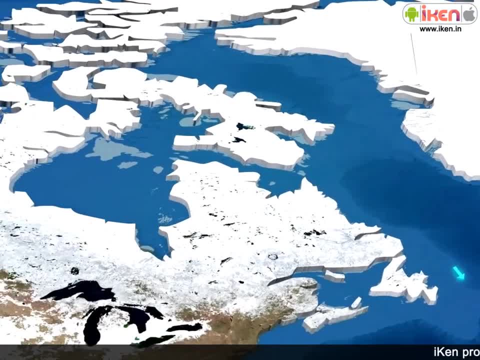 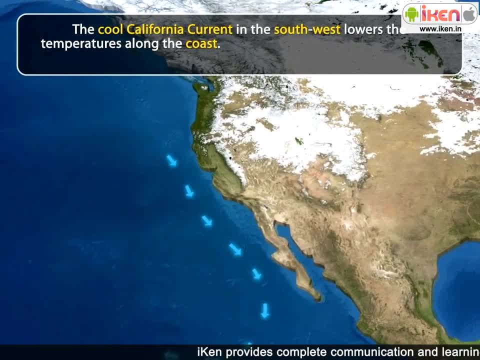 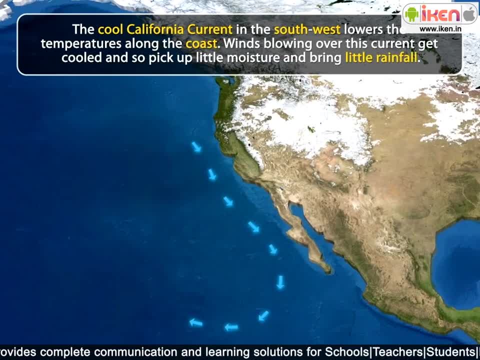 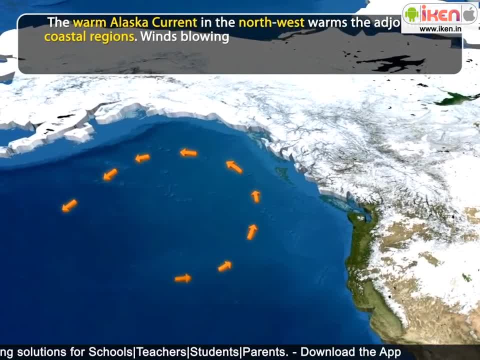 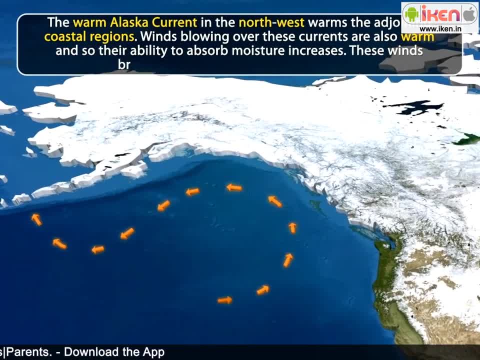 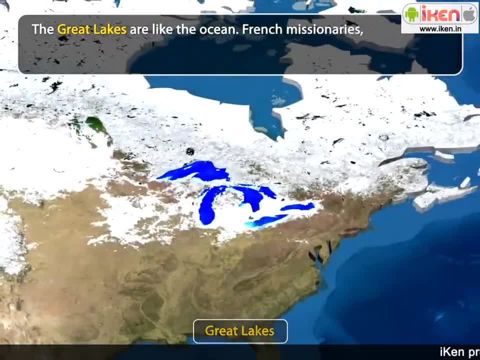 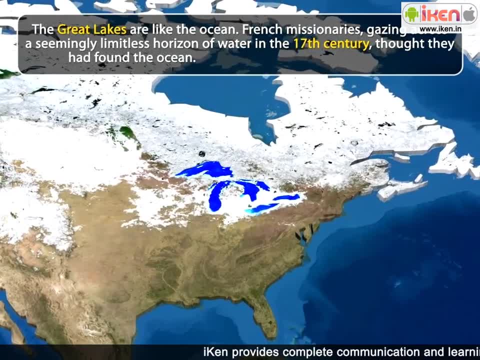 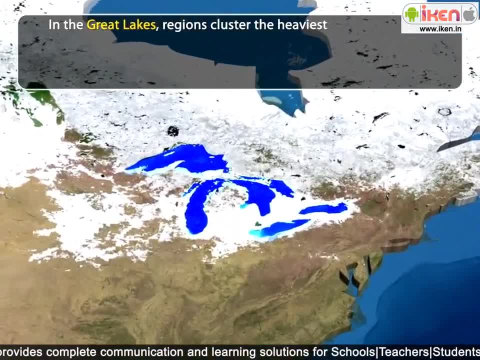 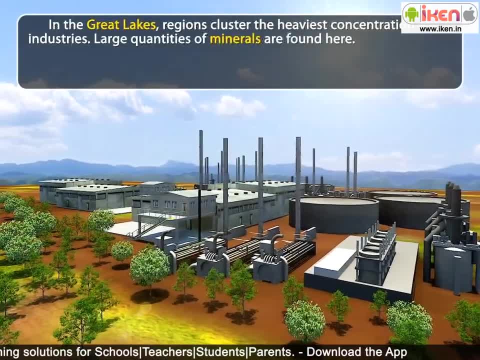 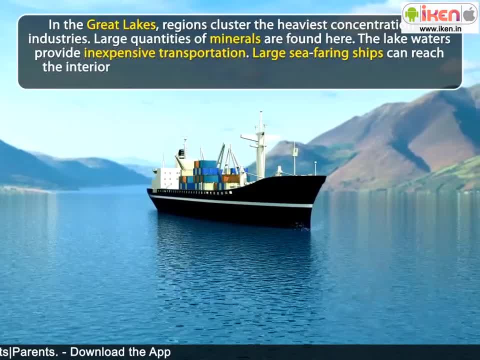 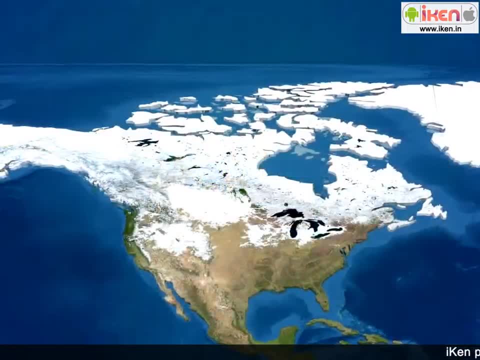 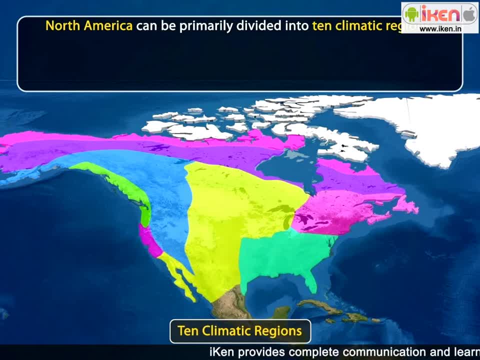 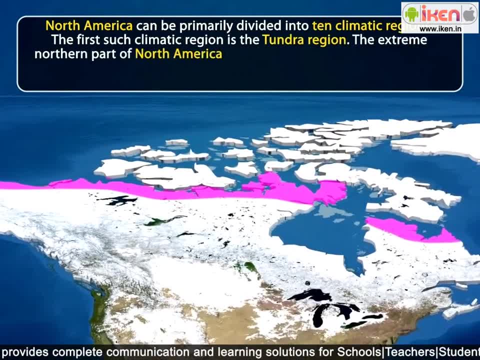 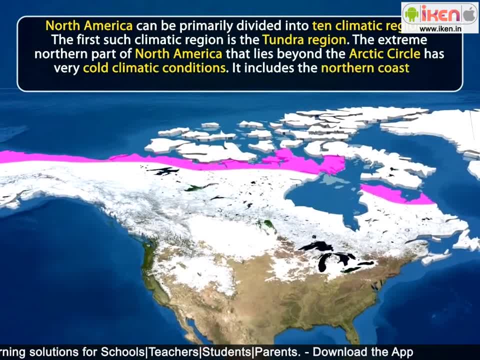 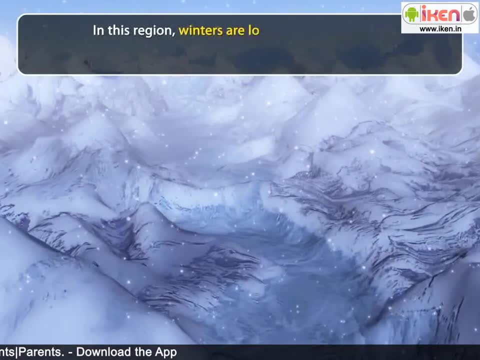 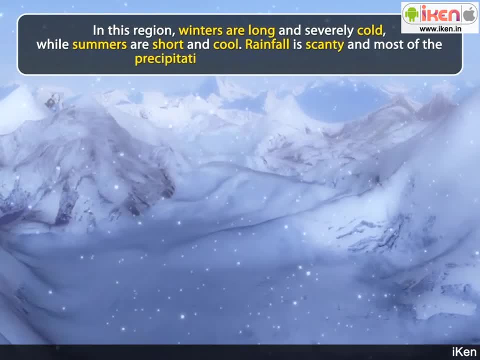 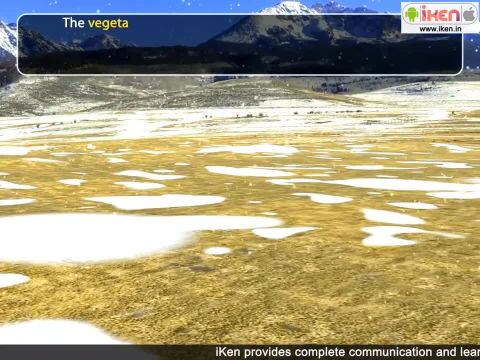 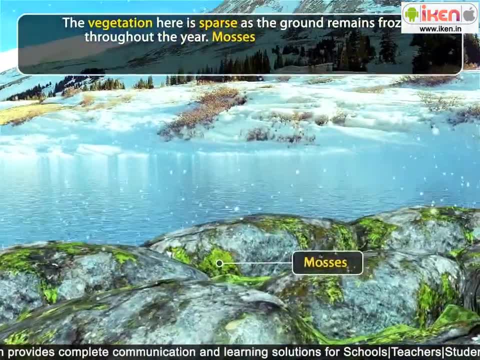 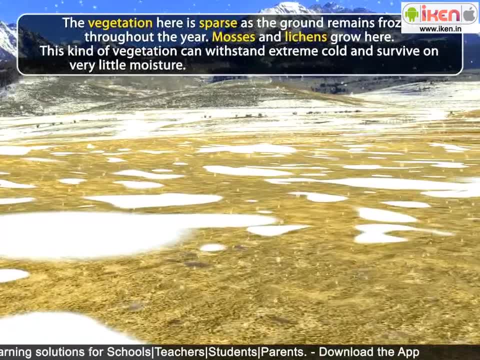 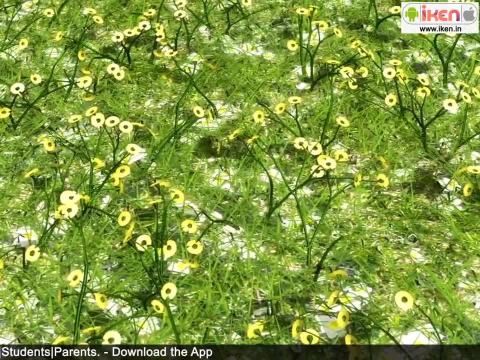 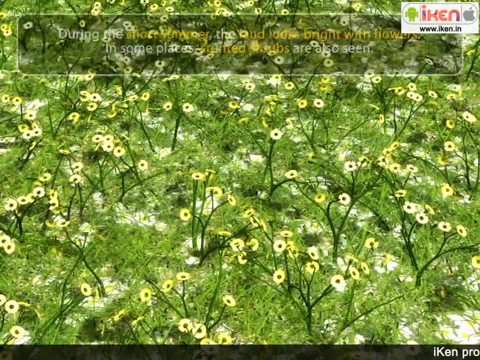 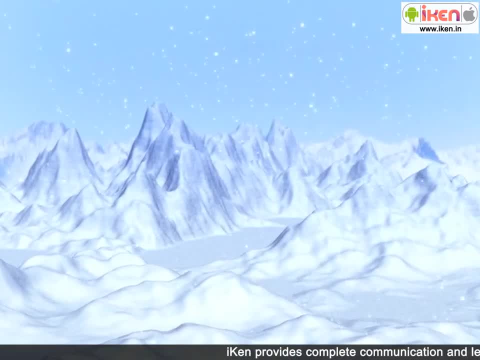 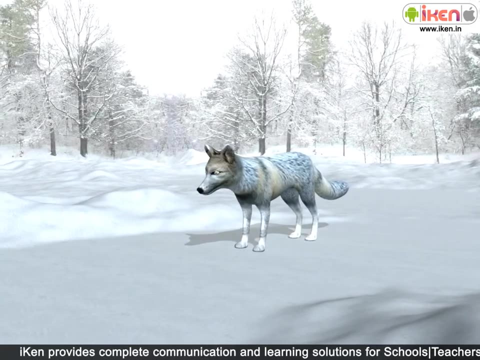 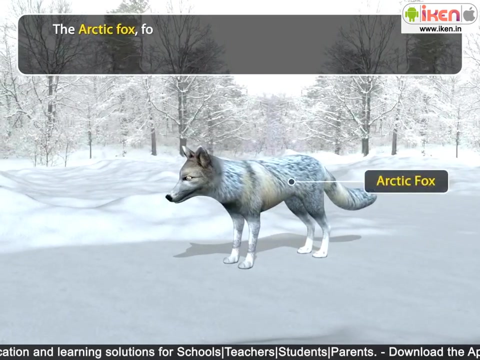 places. stunted shrubs are also seen. Trees cannot grow here because the surface is frozen during winter and the subsoil remains permanently frozen. Animals that are found here usually have thick fur outside and a woolly undercoat to keep them warm. The Arctic fox, for instance, has grey fur in summer, but it turns white in winter. Thick. 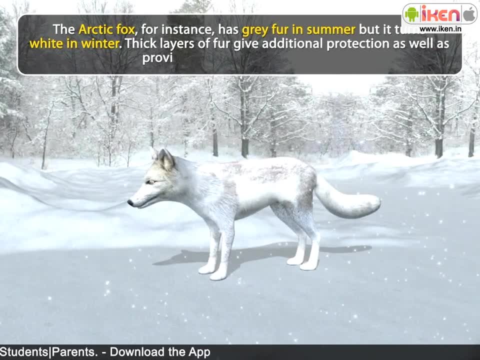 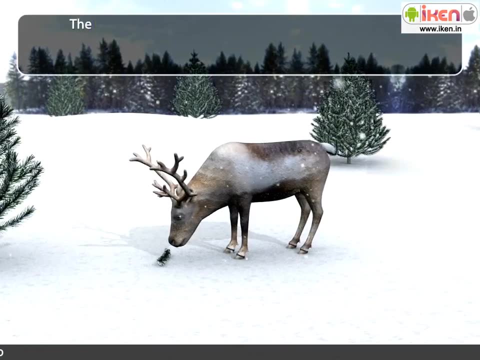 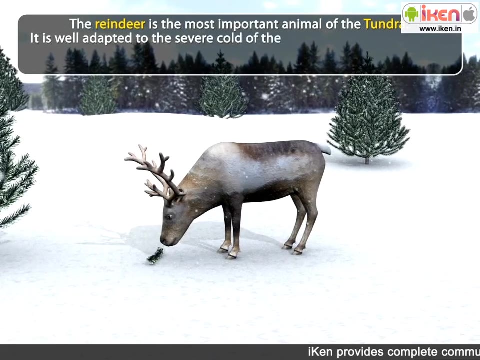 layers of fur give additional protection as well as provide food reserves for winter. The reindeer is the most important animal of the tundra. It is well adapted to the severe cold of the tundra region. Its thick hair and the air cells in each hair makes an excellent protection. 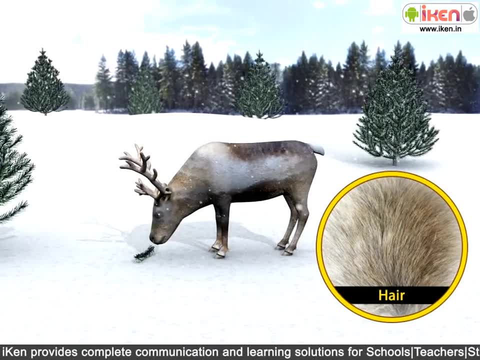 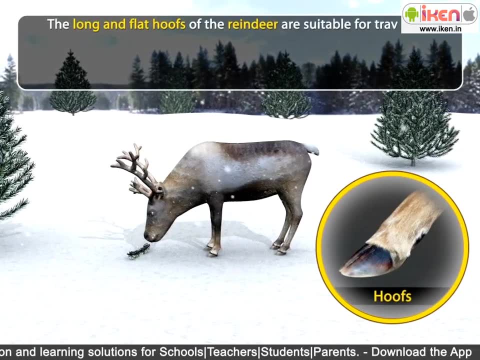 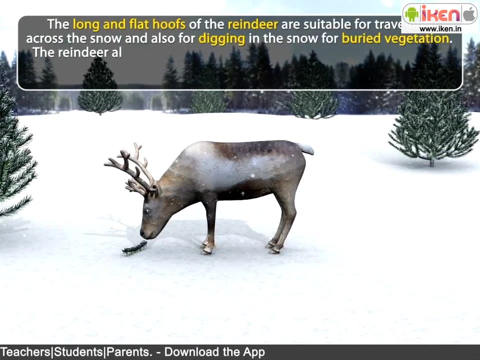 against the cold. The long and flat hooves of the reindeer are suitable for traveling across the snow and also for digging in the snow for buried vegetation. The reindeer also have a good sense of smell and smell. The reindeer are known to have a great sense of smell and smell. Its skin is used for clothing and tents. 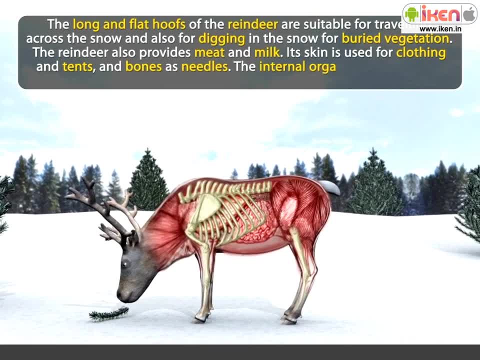 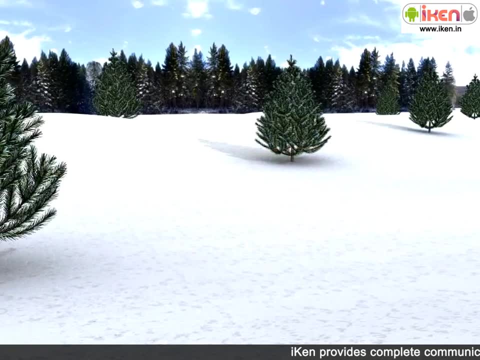 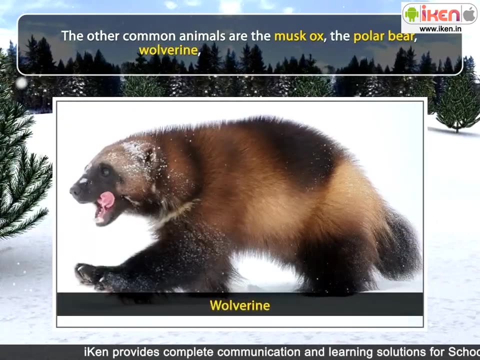 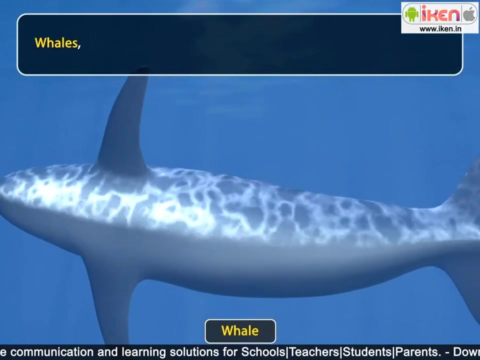 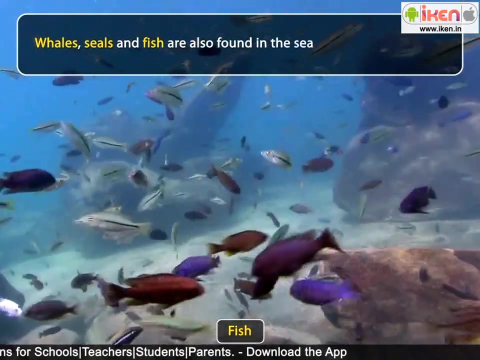 and bones as needles. The internal organs of the reindeer provide vitamins and salts needed by the human body. The other common animals are the musk, ox, the polar bear, Wolverine sable and the blue fox. Whales, Whales, seals and fish are also found in the seas bordering the coast. 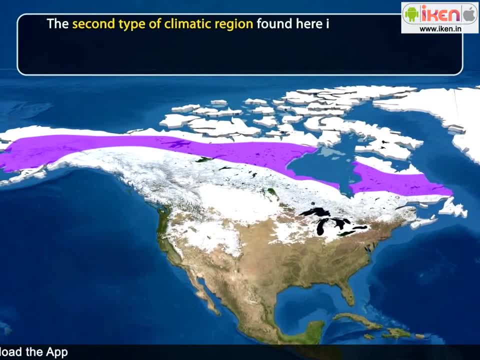 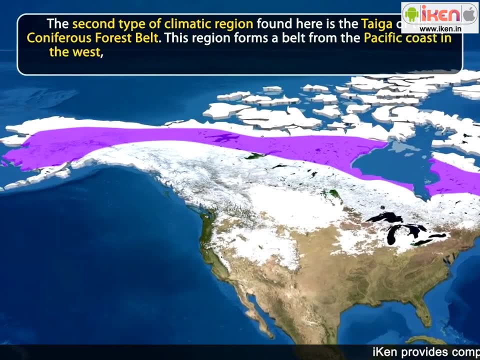 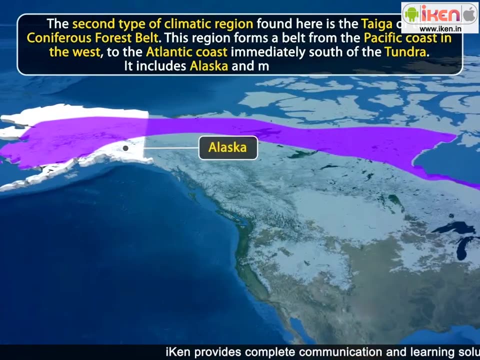 The second type of climatic region found here is the taiga, or the coniferous forest belt. This region forms a belt from the Pacific coast in the west to the Atlantic coast, immediately south of the tundra. It includes Alaska and most of Canada. 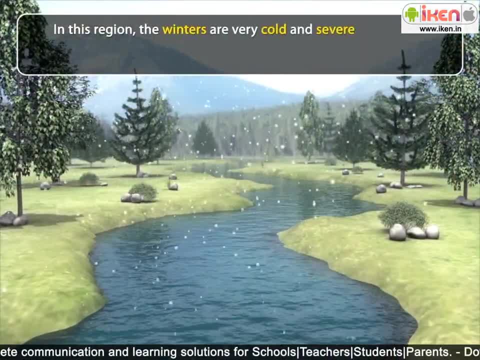 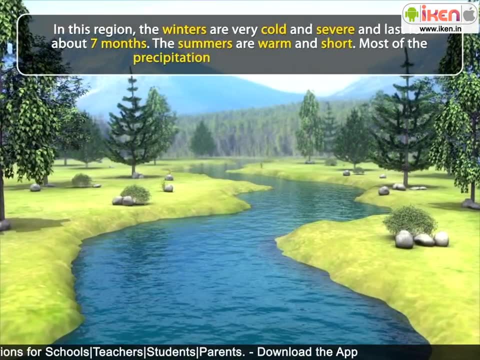 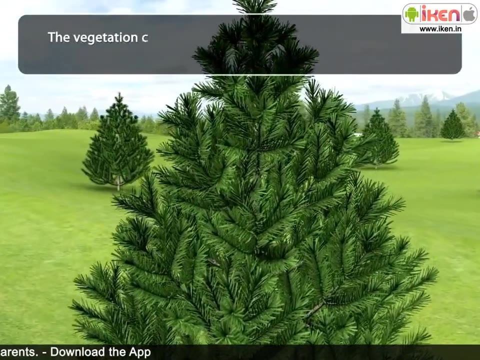 In this region the winters are very cold and severe and last for about seven months. The summers are warm and short. Most of the precipitation is in the form of snow. The vegetation consists of coniferous trees. These are evergreen trees, that is, coniferous trees. 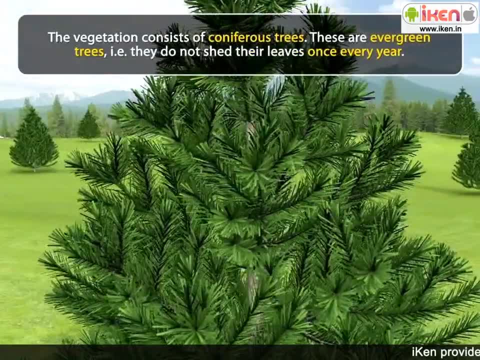 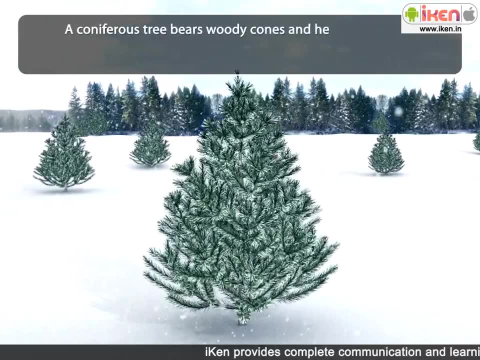 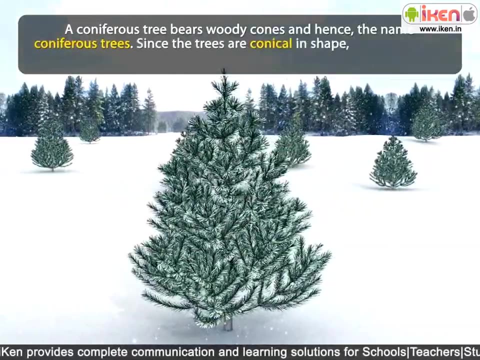 They do not shed their leaves. once every year, A coniferous tree bears woody cones, and hence the name coniferous trees. Since the trees are conical in shape, the snow slides off their branches easily, preventing damage to the trees. 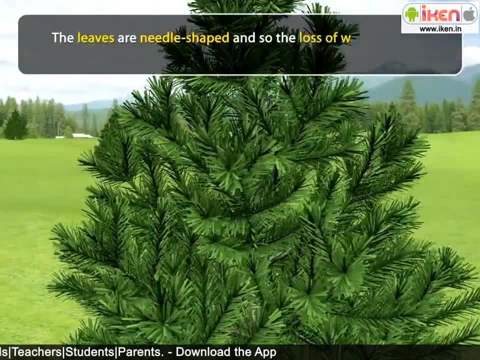 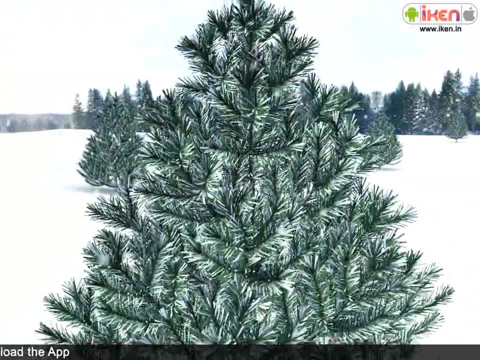 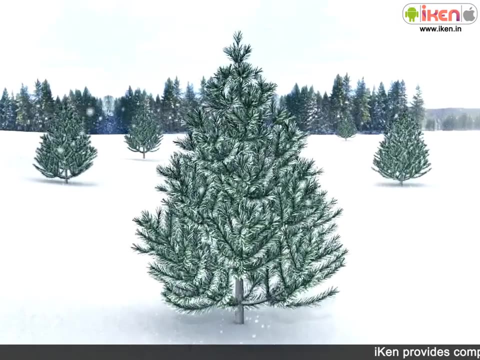 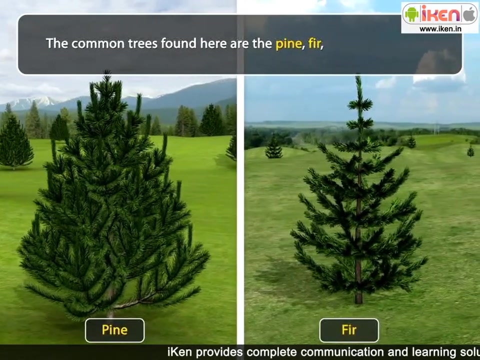 The leaves are needle-shaped, And so the loss of water through evaporation is reduced, since the surface area of the leaf is reduced, Hence they are able to survive the long winter when the water is frozen and not easily available. The common trees found here are the pine fir, cedar and spruce. 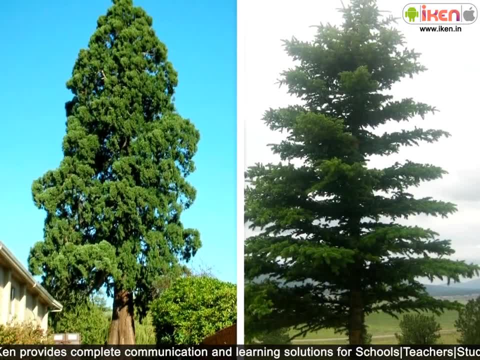 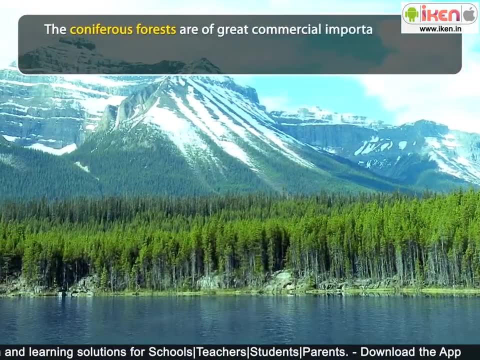 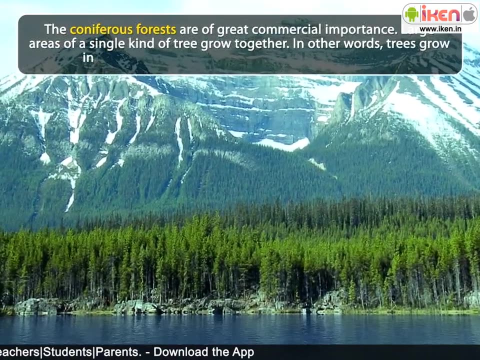 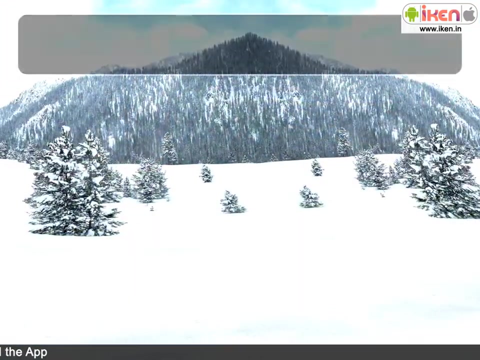 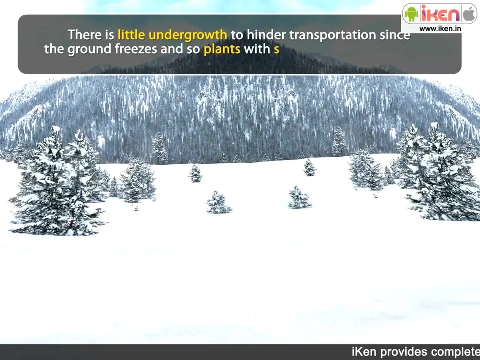 They are adapted to survive the severe, long winters. The coniferous forests are of great commercial importance. Large areas of a single kind of tree grow together, In other words, trees grow in social strands, making lumbering operations easy. There is little undergrowth to hinder transportation, since the ground freezes, and so plants with short roots cannot survive. 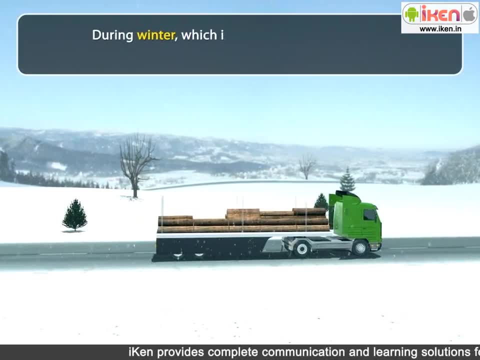 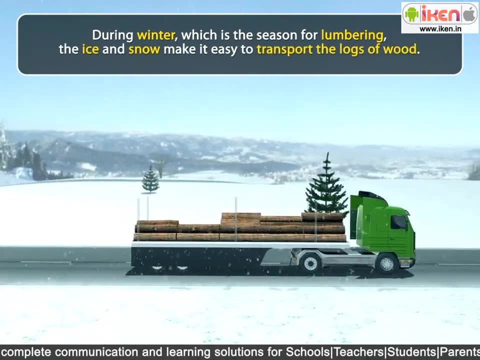 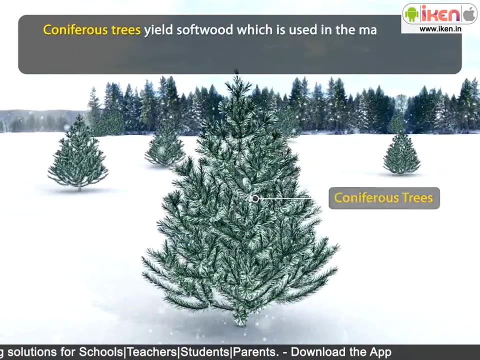 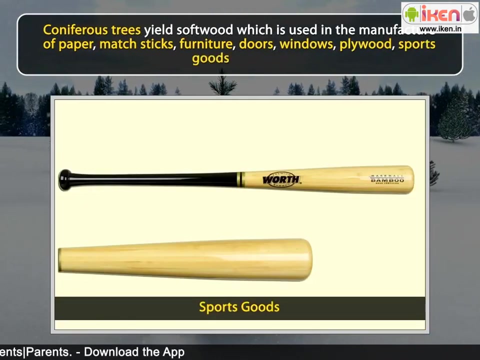 During winter, which is the season for lumbering the ice and snow make it easy to transport the logs of wood. Coniferous trees yield soft wood which is used in the manufacture of paper, matchsticks, furniture, doors, windows, plywood, sports goods and toys. 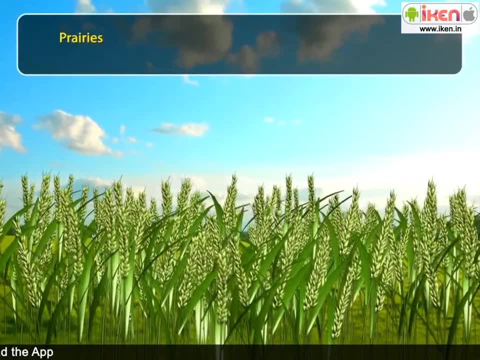 The trees are used to transport land, food and other machinery, and they are also used for transportation. The area of the forest can be used for mining. There are해�木 and wood, a gold mine, a cole jar and a small way of commerce for the dyke. 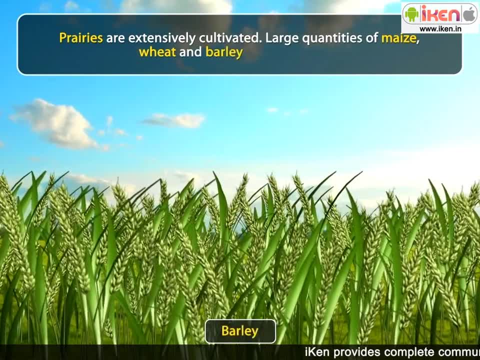 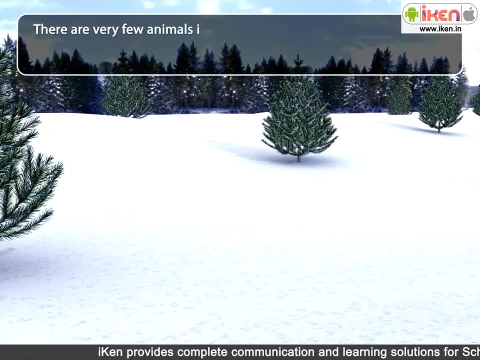 The main, primary part of wood production is the manufacturing of a wood plant which is said to have a meat knack. It is the local. There are very few animals in this region and most of them are small. The beaver, fox, sable, ermine, skunk and raccoon yield fur. The best fish and animals to be grown in this region are the flounder, the ogre, the snake, the magpie, the spider, the fox or the wax moth. They are above the nimbler, the snake, the hawk, the carpenter and the moth. 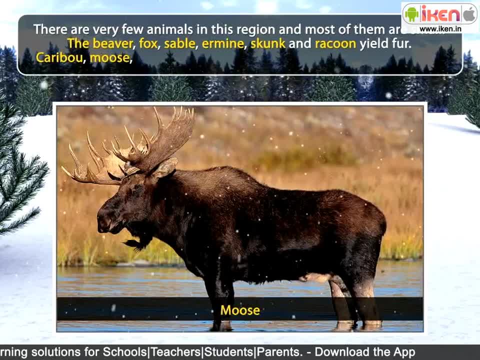 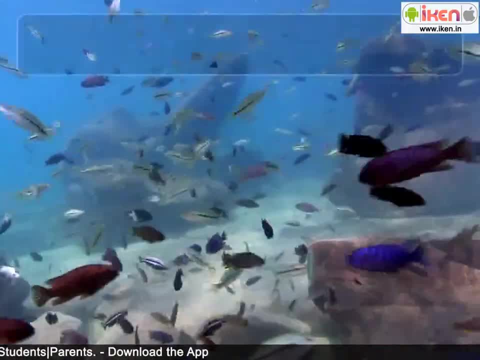 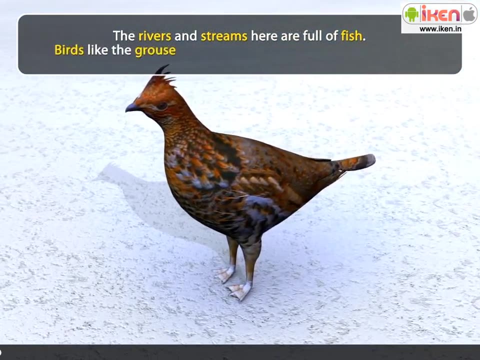 They are the most powerful animals to be grown in this area. fur, caribou, moose, elk and brown, black and grizzly bears are common. The rivers and streams here are full of fish. Birds like the grouse and the woodpecker are also found.